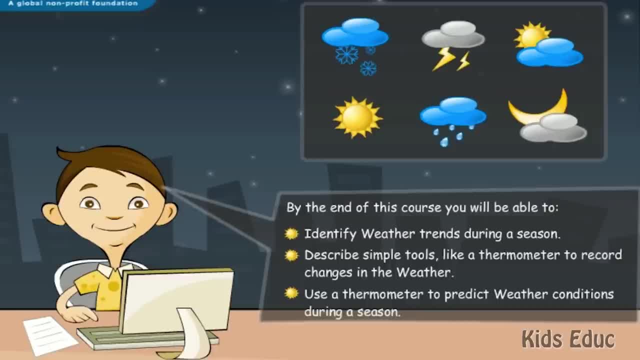 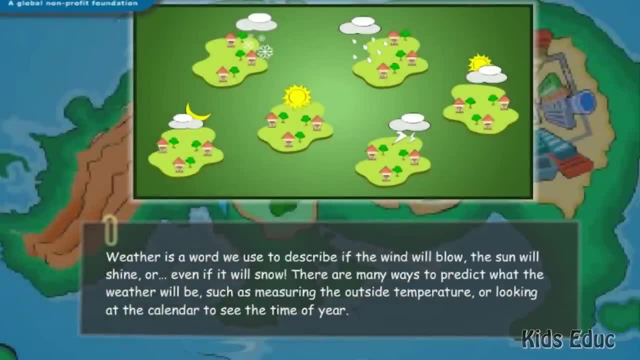 Use a thermometer to predict weather conditions during a season. Are you ready to begin? Weather is a word we use to describe if the wind will blow, the sun will shine or if the weather is bad. There are many ways to predict what the weather will be. 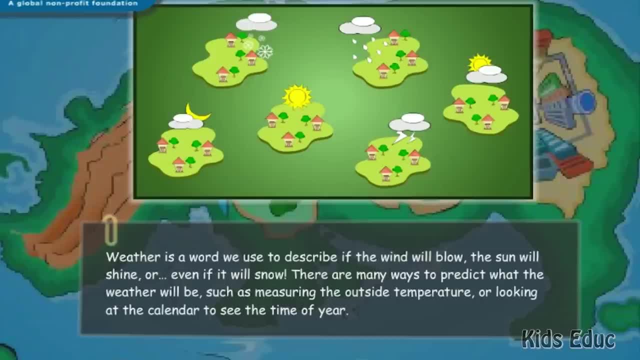 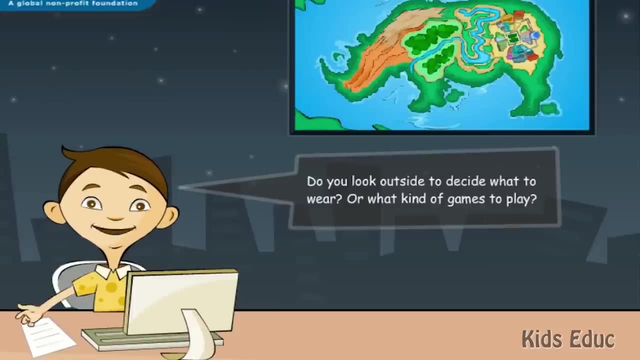 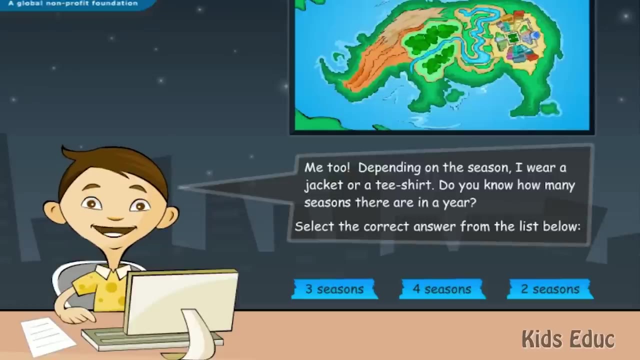 such as measuring the outside temperature or looking at the calendar to see the time of year. Do you look outside to decide what to wear or what kind of games to play? Me too. Depending on the season, I wear a jacket or a t-shirt. 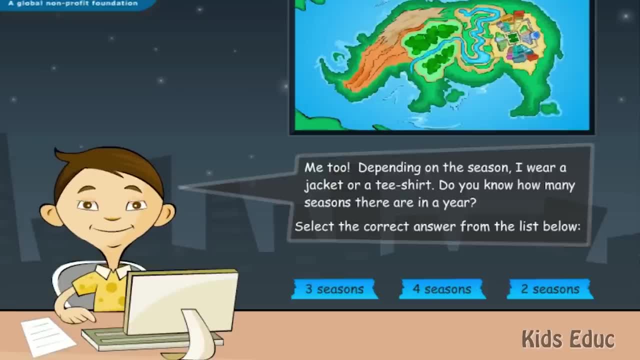 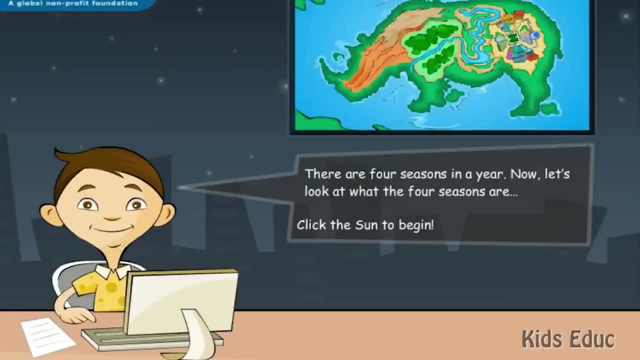 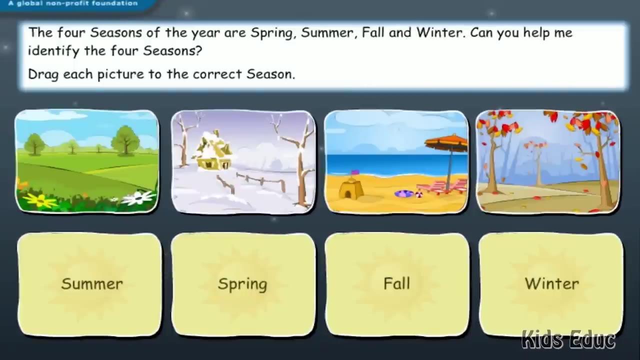 Do you know how many seasons there are in a year? The correct answer is four seasons, Correct: There are four seasons in a year. Now let's look at what the four seasons are. The four seasons of the year are spring, summer, fall and winter. 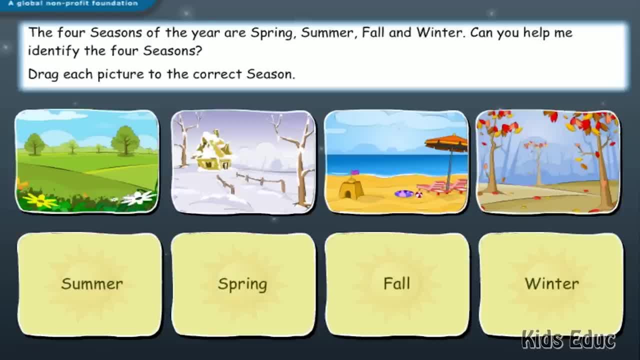 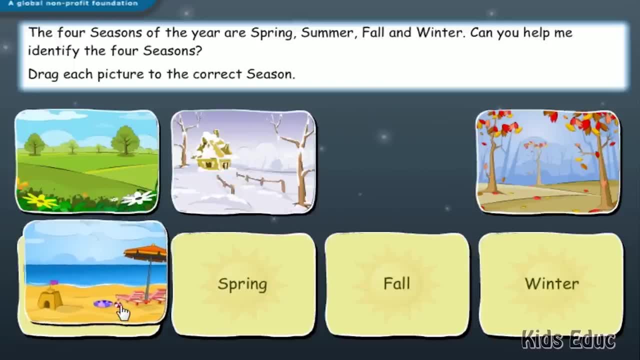 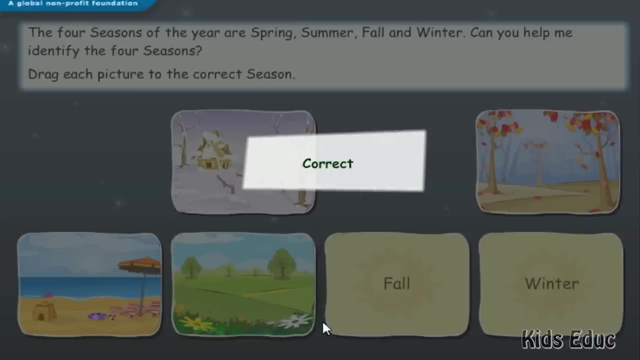 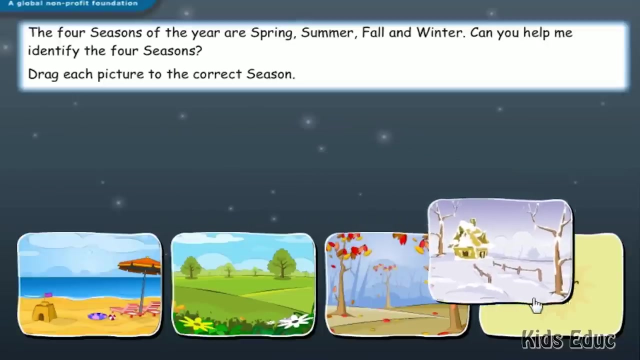 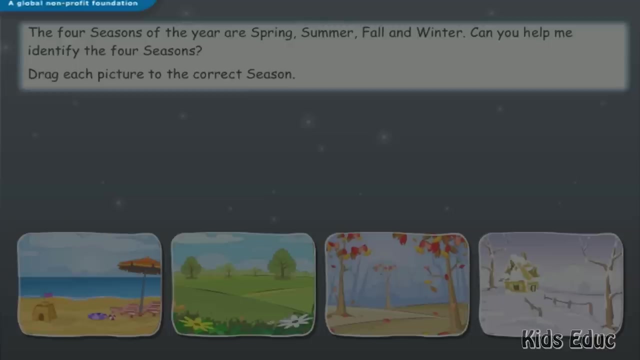 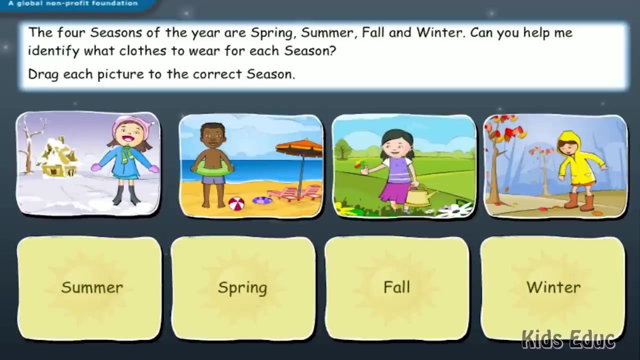 Can you help me identify the four seasons? Drag each picture to the correct season. Correct, That was easy, wasn't it? Now let's find out what clothes we can wear for each season. Can you help me identify the clothes to wear for each season? 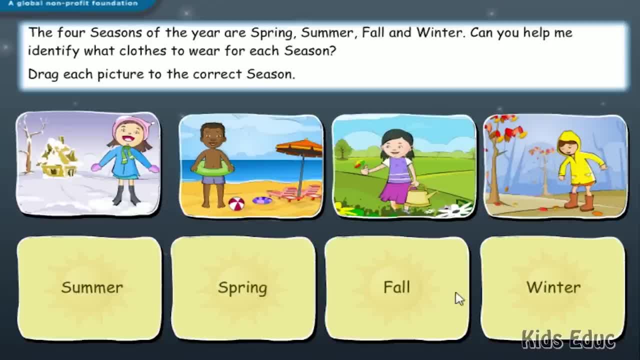 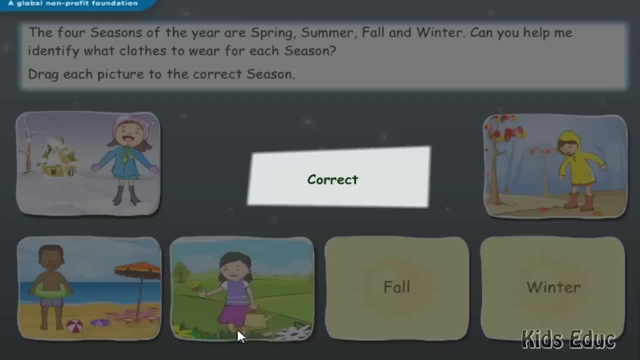 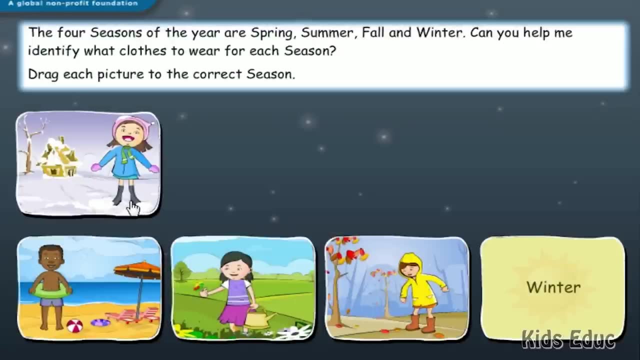 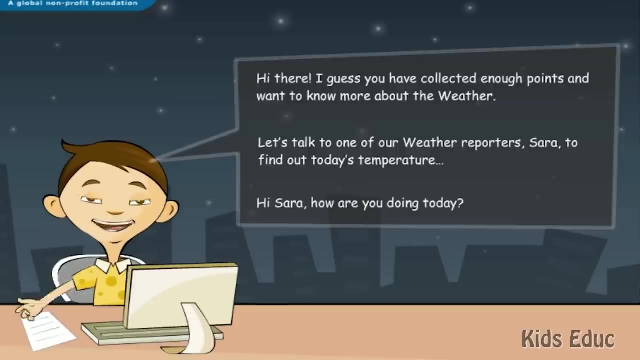 Drag each picture to the correct season. Correct, Correct, Correct, Correct. Hi there, I guess you have collected enough points and want to know more about the weather. Let's talk to one of our weather reporters, Sarah, to find out today's temperature. 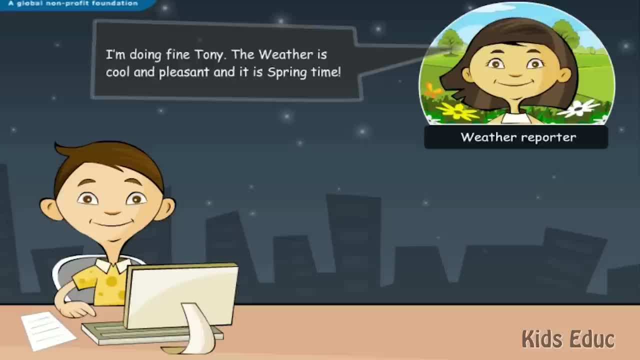 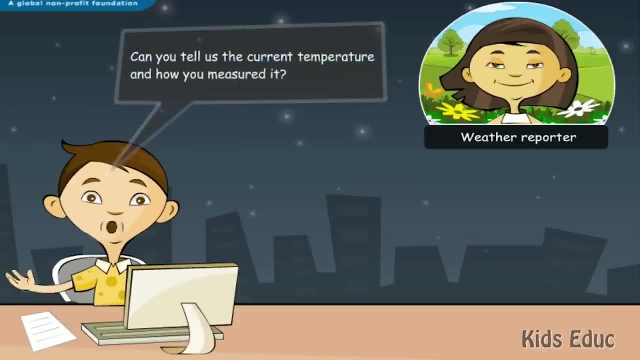 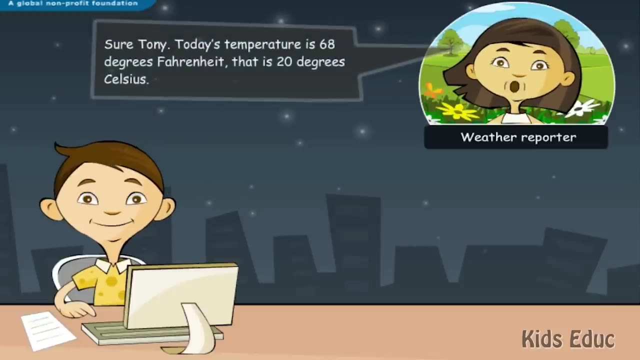 Hi Sarah. how are you doing today? I'm doing fine, Tony. The weather is cool and pleasant and it is springtime. Can you tell us the current temperature and how you measured it? Sure, Tony, Today's temperature is 68 degrees Fahrenheit, that is, 20 degrees Celsius. 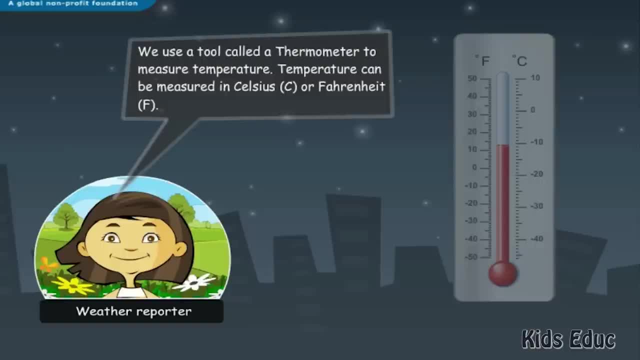 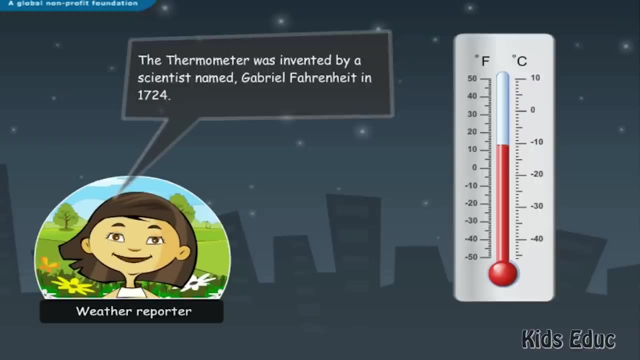 Let's find out how to measure temperature. We use a tool called a thermometer to measure temperature. Temperature can be measured in Celsius or Fahrenheit. The thermometer was invented by a scientist named Gabriel Fahrenheit in 1724.. Let's see how it works. 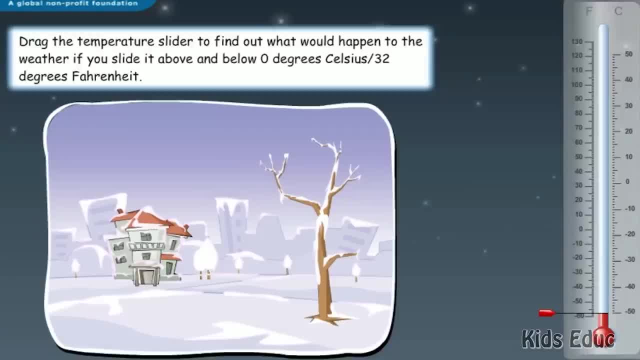 Drag the temperature slider to find out what would happen to the weather if you slide it above and below zero degrees Celsius, 32 degrees Fahrenheit. OK, Let's see how it works. Let's see how it works Winter, Winter, Winter. 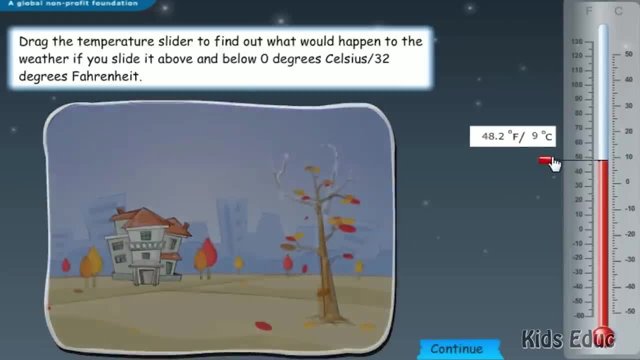 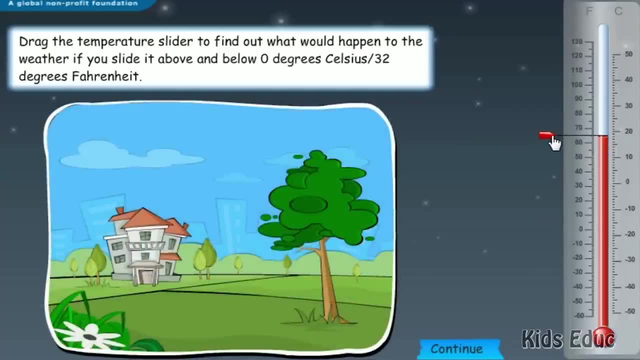 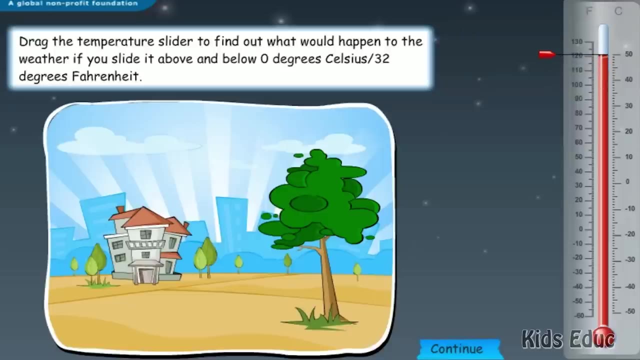 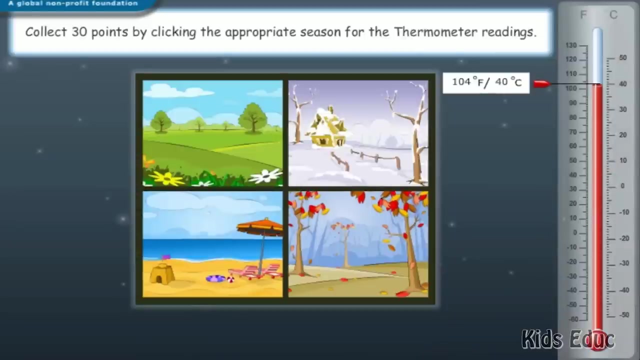 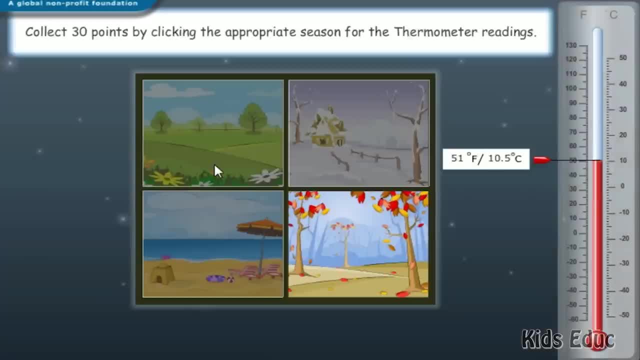 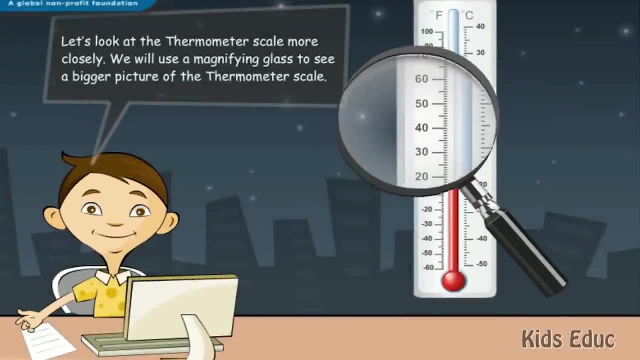 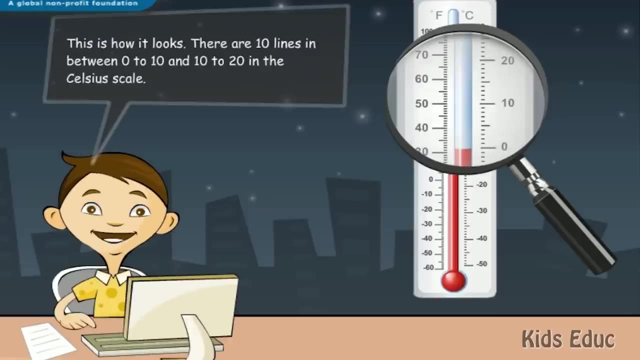 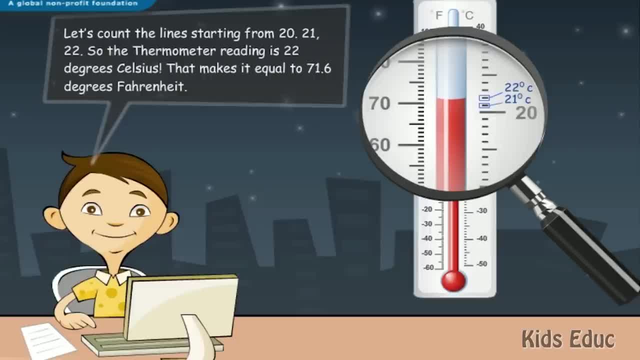 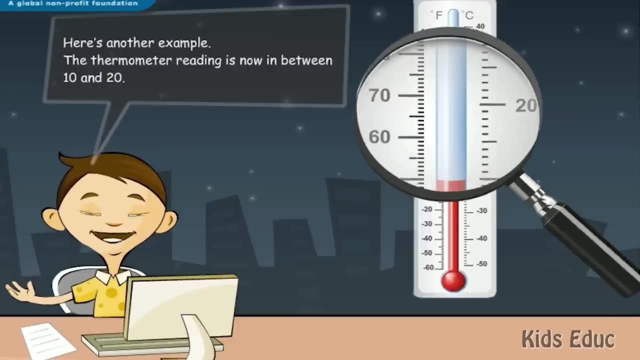 Let's count the lines starting from 20,, 21,, 22.. So the thermometer reading is 22 degrees Celsius. That makes it equal to 71.6 degrees Fahrenheit. Here's another example. The thermometer reading is now in between 10 and 20.. Let's count the lines starting from. 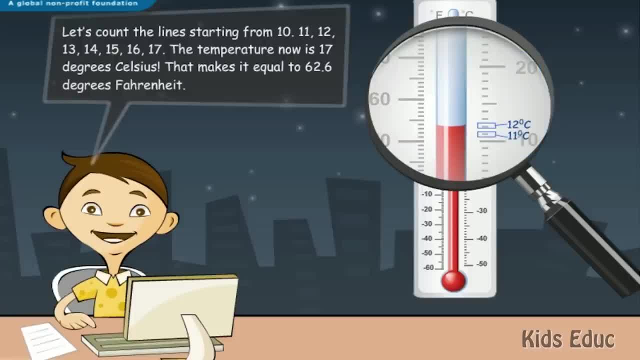 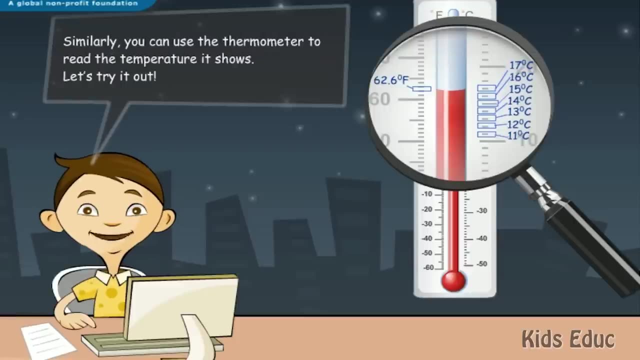 10,, 11,, 12,, 13,, 14,, 15,, 16, 17.. The temperature now is 17 degrees Celsius. That makes it equal to 62.6 degrees Fahrenheit. Similarly, you can use the thermometer to read the temperature it shows. Let's try. 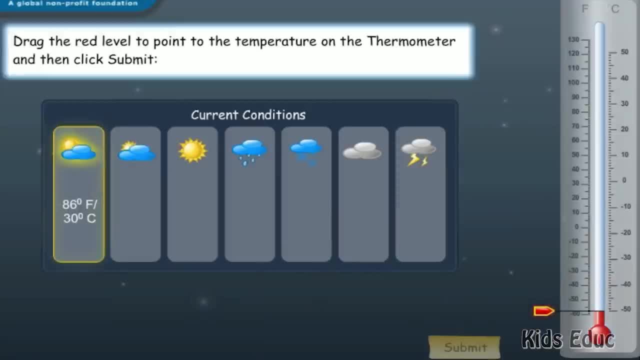 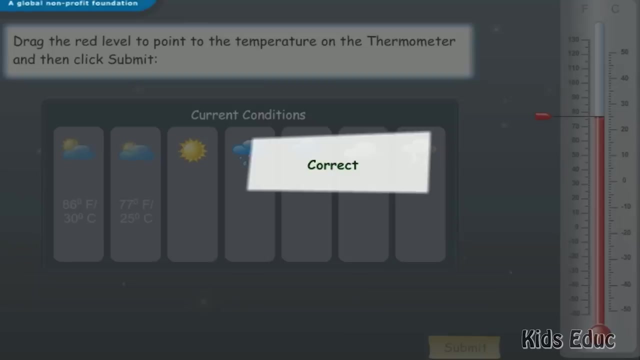 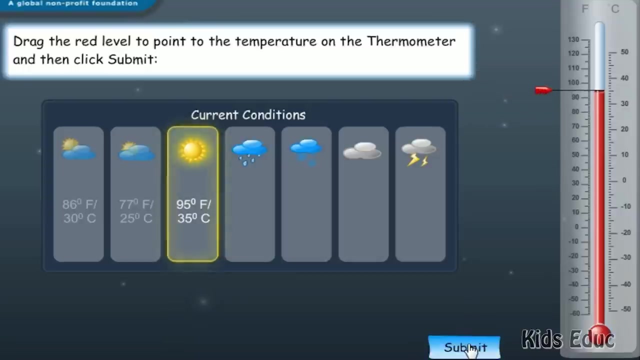 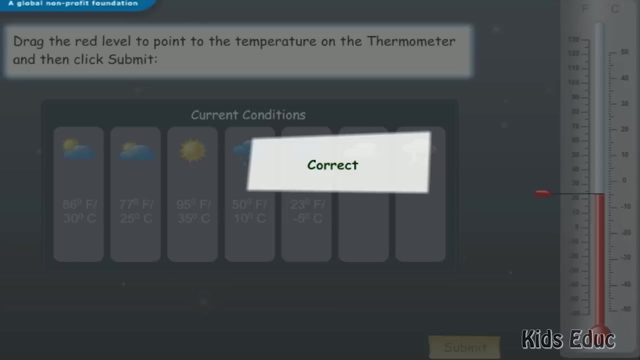 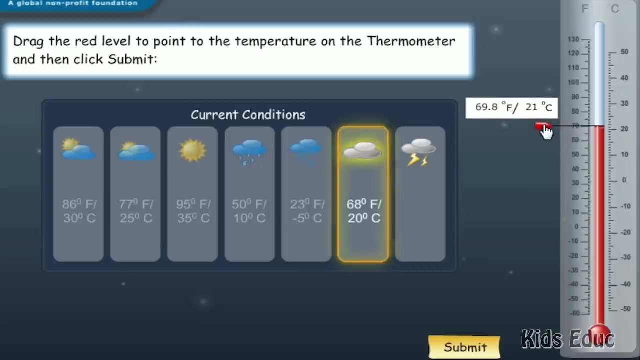 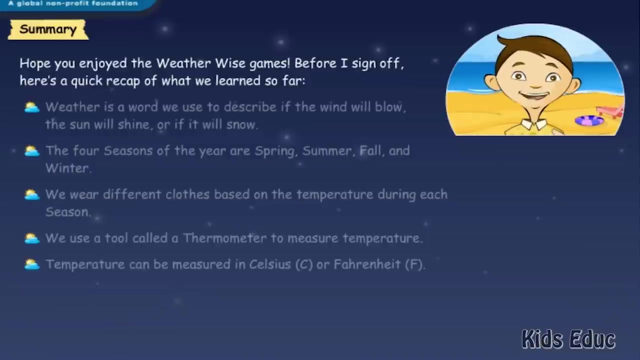 it out. Drag the red level to point to the temperature on the thermometer and then click Submit. Correct, Correct, Correct, Correct. Hope you enjoyed the WeatherWise games. Before I sign off, here's a quick recap of what we've learned so far. 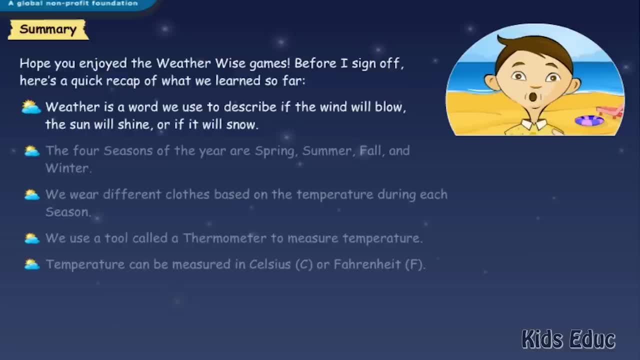 Weather is a word we use to describe if the wind will blow, the sun will shine or if it will snow. The four seasons of the year are spring, summer, fall and winter. We wear different clothes based on the temperature during each season. We use a tool called a. 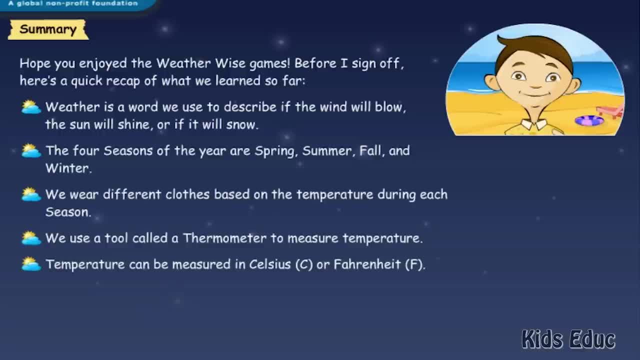 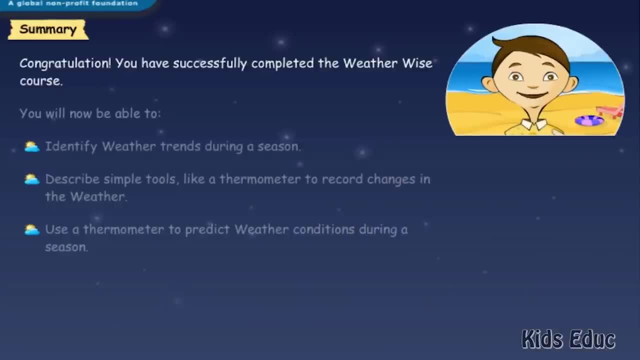 thermometer to measure temperature. Temperature can be measured in Celsius or Fahrenheit. Congratulations, You have successfully measured the temperature of your home. You can now use a thermometer to measure the temperature of your home. You will now be able to identify weather trends during a season. describe simple tools like a thermometer to record. 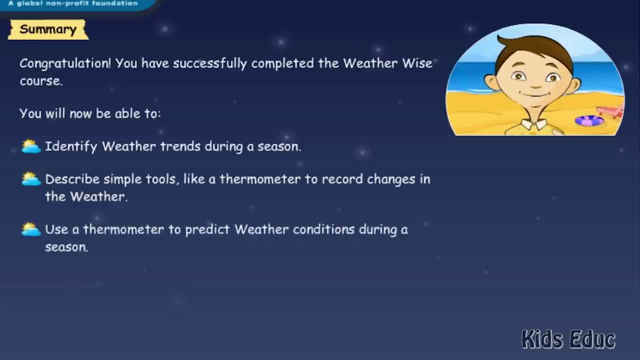 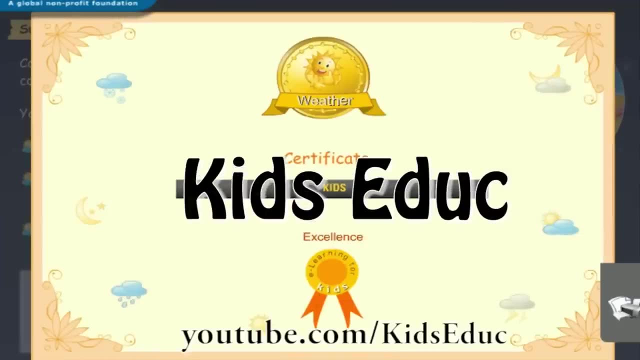 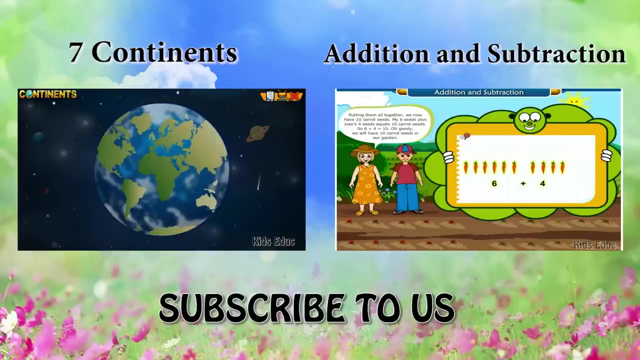 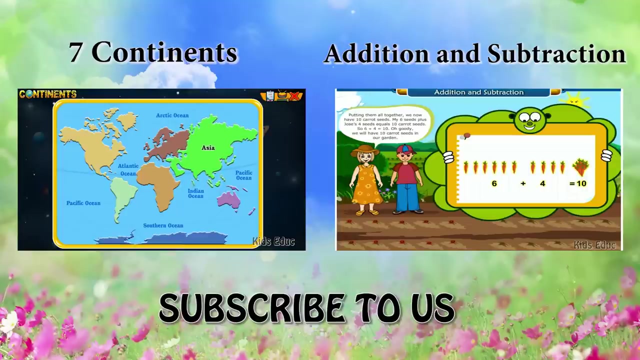 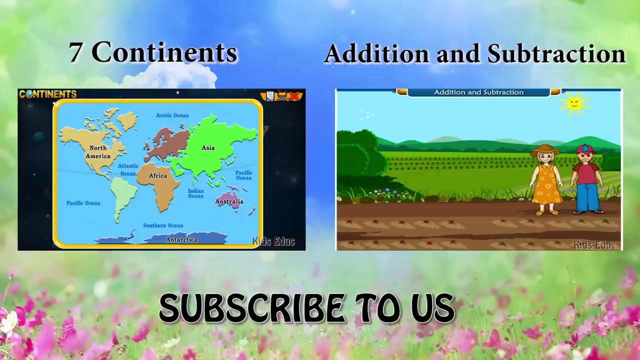 changes in the weather. use a thermometer to predict weather conditions during a season. and use a thermometer to measure weather conditions during a season. Thank you.